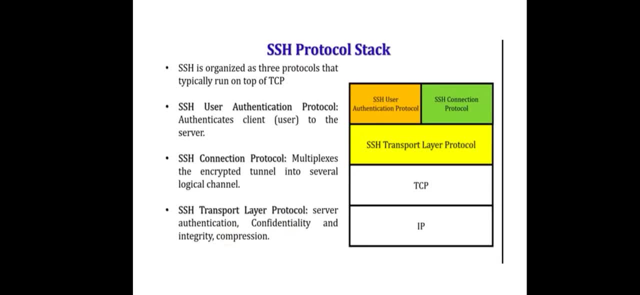 file transfer and email And SSH protocol stack. SSH is organized as three protocols that typically run on top of TCP: SSH User Authentication Protocol, SSH Connection Protocol, SSH Transport Layer Protocol. So Secure Cell chooses combination of three protocols that typically run on the transport layer. First protocol is Secure Cell User Authentication Protocol. 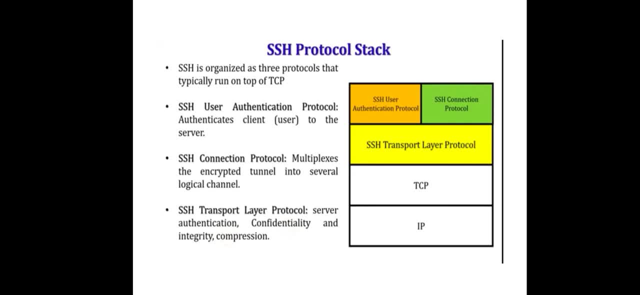 First protocol is Secure Cell User Authentication Protocol. Name suggests itself. this protocol is used for authentication, So it is responsible for authenticates clients to the server. And the second protocol is Secure Cell Connection Protocol. It is responsible to create encrypted tunnel into several logical channels. 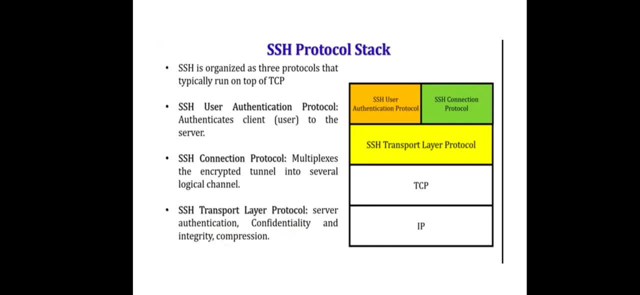 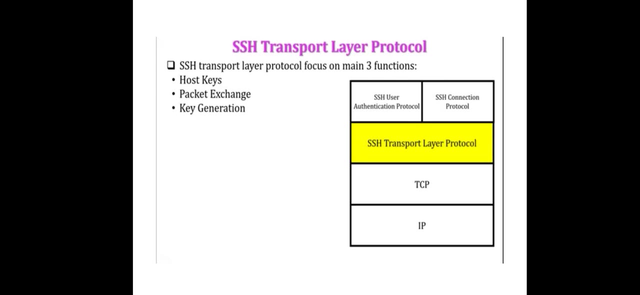 And third protocol is Transport Layer Protocol. It is responsible for several server authentication, data data confidentiality, etc. data integrity and data comprehension. so in this SSH transport layer protocol we are having three main focus, three main functions. first one is host key. second one is packet exchange and third one is key generation. so the first one, host. 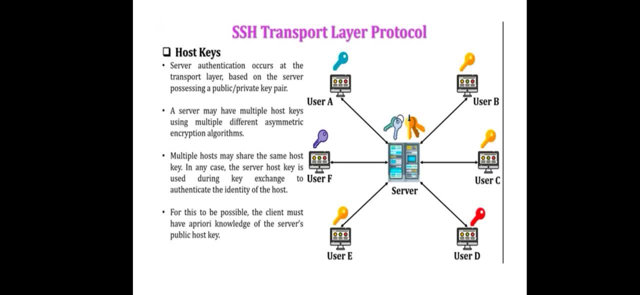 keys. server authentication occurs in the transport layer based on the server process processing a public or private pay. a server may have multiple host keys using multiple different asymmetric encryption algorithms. multiple hosts may say the same host key. in any case, the server host key is used during key. 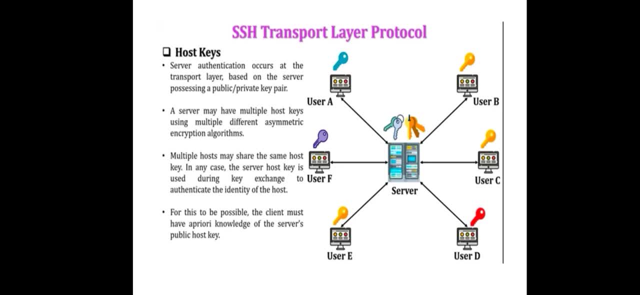 exchange to authenticate the identity of the host. for these to be possible, the client must have appropriate knowledge of the server public host key. so in host key client must know about server public host keys for the key exchange. to alternate to TRUST models that can be used in first, that can be used and. 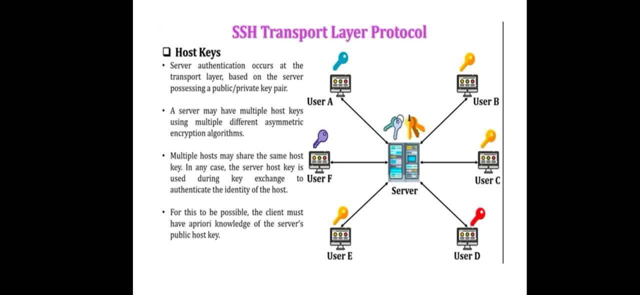 first, more first, model is the client that has a local database. all the clients have to connect with that local database and the local database store each host name with the corresponding host case and the second one is the hostname to key association and it is verified by a certificate authority. 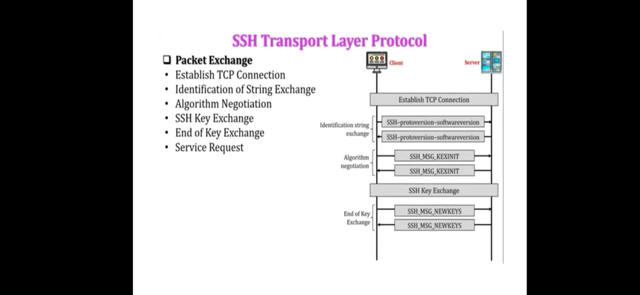 next one is packet exchange. in packet exchange we are having six steps. first is establish tcp connection. second is identification of string exchange: studies, algorithm negotiations for these secure key exchange. fifth is end of key exchange and 60 service request. there is a client and a server. first in, in first client, establish a tcp connection to the server. 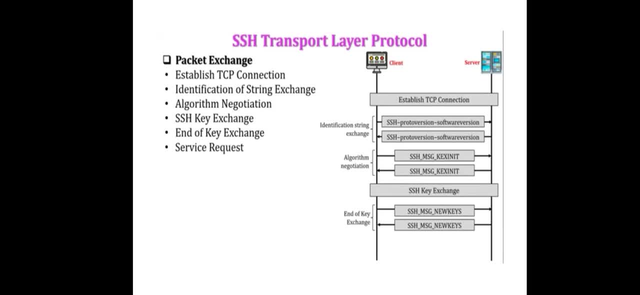 this is done by the tcp protocol and it is not a part of the secure transport layer protocol. once a connection is established between the client and the server, then client and the server exchange the tcp connection to the server, the data it is exchange, the data it is referred as to be packet and transport. 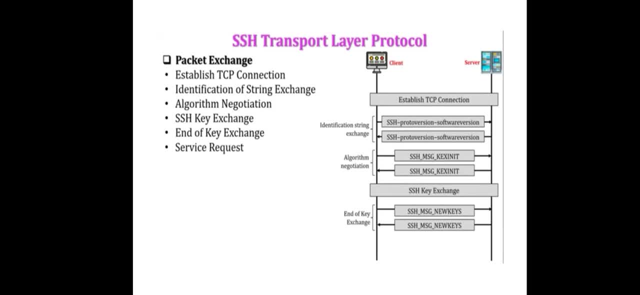 layer package exchange constitutes of a sequence of steps. the first one is identification of string exchange. it begins with the client sending a packet with an identity identification string to begins, with the client to the string, and next step is algorithm negotiation. in this step, client and servers send and. 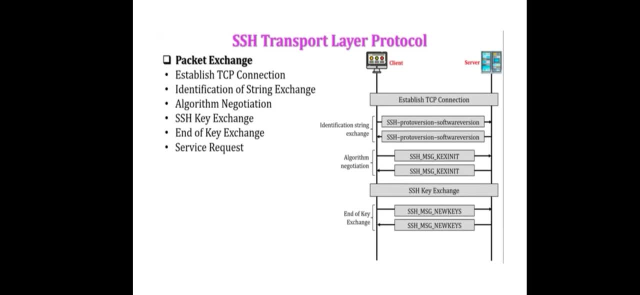 secure cell message: key exchange initialization. this message contains a list of supported algorithm and the next step is secure cell key exchange. if we help an algorithm, it is used for the key exchange and the next one is the end of the key exchange. the end of the key exchange is signaled by the exchange off secure cell. 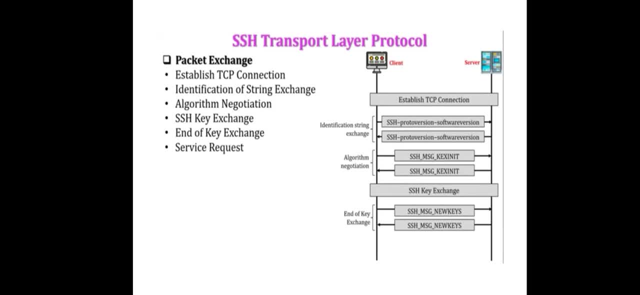 message: new key packets. at the point, both sides may start using key generations from the master key and the final step is packet exchange. it is a service request. in this step, client sends a service request. either they use the authentication or the Centauri if the machine is. 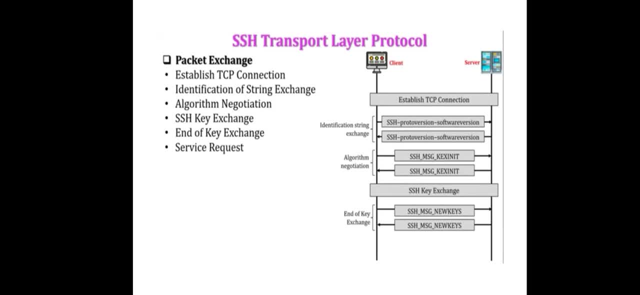 still on. we will. the service request that is I kept in the past because I don't know the talk that I didn't send. a last step connection issues. I have the key of the master key and protocol. after that, all the data is exchanged which is protected by the. 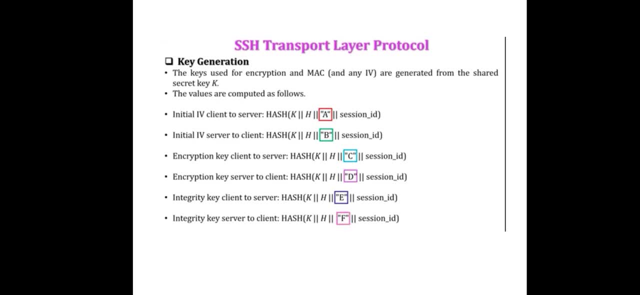 encryption and the next one is key generation. in transport layer protocol the keys used for encryption and the MAC and any initial vector are generated from the shared secret key K. so the values are computed as follows. first one: it initial initial from client to server. here the key generated values are: 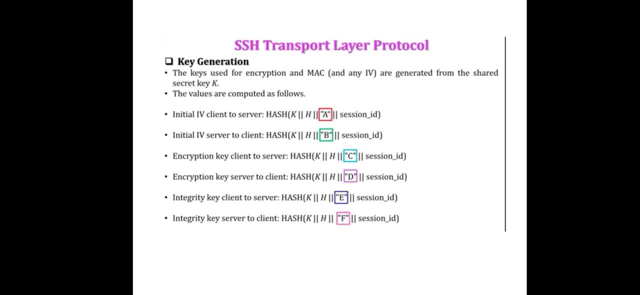 calculated as K, K as secret key, H as host value from the key exchange and the value A is generated from the secret key K and the session ID indicates the session identifier and second one initial from server to client. here K is the secret key, H is Kü. Speaker 5. 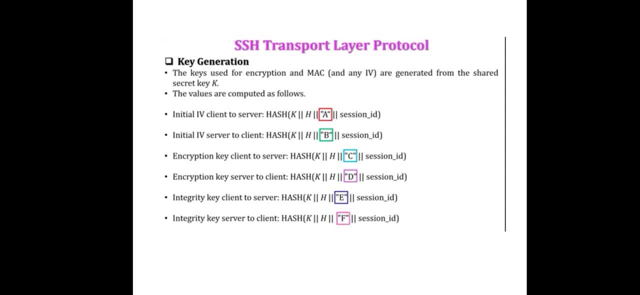 hash value from the key exchange and the value B is generated from the secret key K and the session ID indicates the session identifier and here the encryption key from client to server. here K is the secret key, H is the hash from the key exchange and the value C is generator from the secret key K and the. 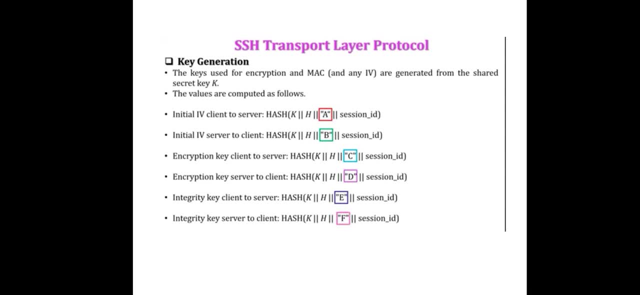 session ID indicates the session identifier and here encryption key from server to client. same as k is secret, h is hash value, d is a generated from secret key, k and integrity key from client to server. here he is also generated from the secret key and f is also generated from the. 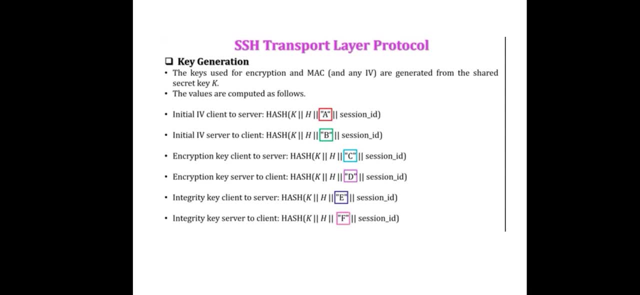 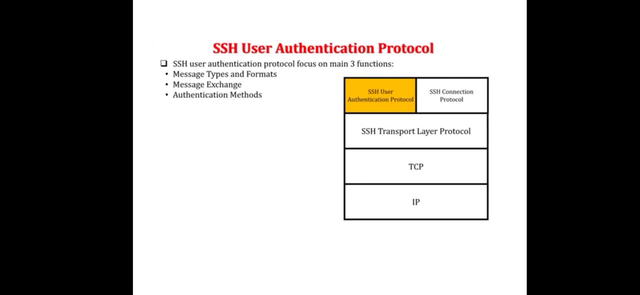 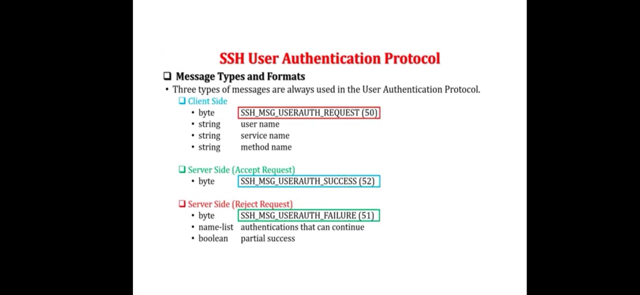 secret. these f is generated from the sequent key in integrity key: server to client. now next is ssh user authentication protocol. ssh user authentication protocol- ssh user authentication. authentication protocol has three main functions. first one is message types and formats. second one is message exchange. start is authentication method. so from the first one message type and formers from: 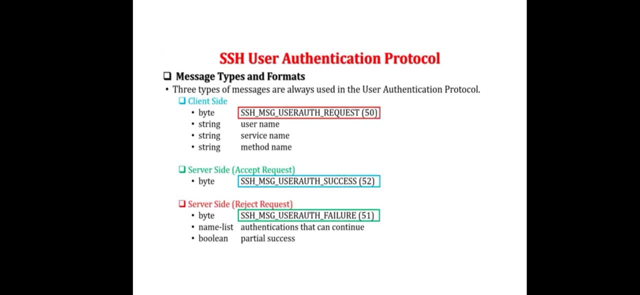 these three types of messages. there are three types in the authentication protocol and in these three type of message. first message is used by client side. the messages use these messages: youth user authentication request. this message is sent by the client to the server. this message includes username, service name and method name after clients a request. after client request. 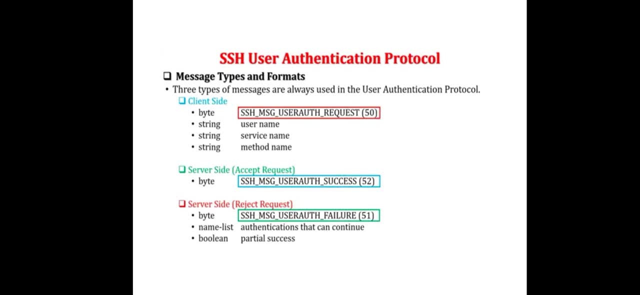 message. if the server accept the authentication, it sends a single byte message. this message: is user authentication successful here, the 50 indicates that it is requesting. it is requesting and the 52 indicates that the user authentication is successful at the server side. if the server rejects the authentication request, then server sends: 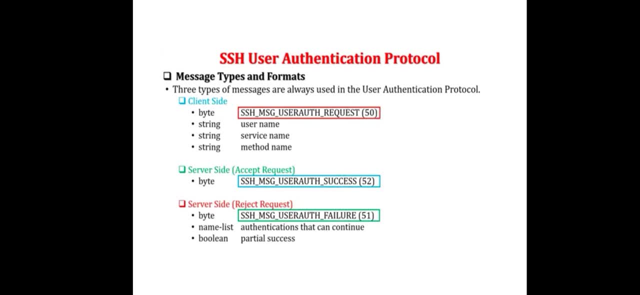 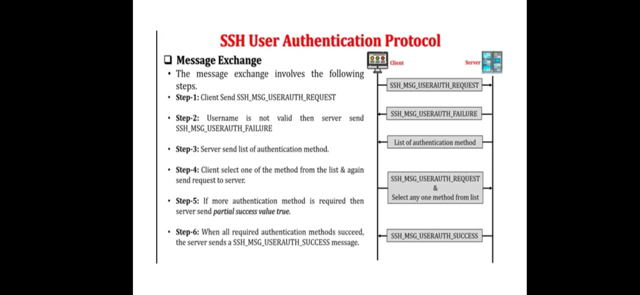 a message: you user authentication failure to the client. so in this function these three types of messages are always used, and here the 51 indicates its failure. the user authentication is failure and the next one is this message exchange. the message exchange involves the following strip: step one is clients, since secured cell message, user authentication request and. 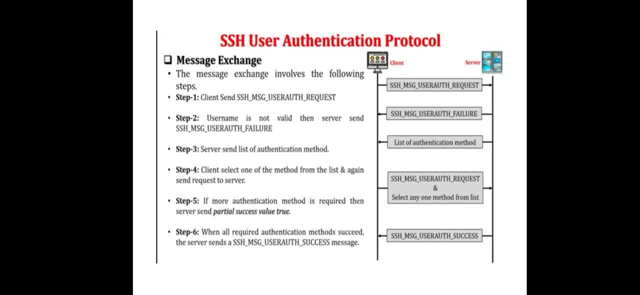 username is not valued, then serve us. and user server send secured cell message. user user authentication failure. that step is server seen list of authentication method. four step is clients select one of them, a third, from the list and again. and 5th step is: if more authentication method is required, then server send partial success. 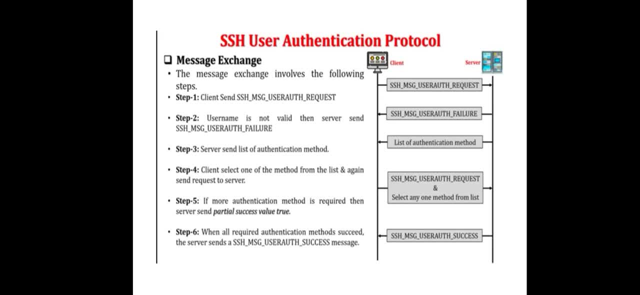 value true. 6th step is when all required authentication method succeed. then the server sends a secure cell message. user authentication success message. lets see in message exchange it takes between the client and a server and the first step is the client sends user authentication request to the server. 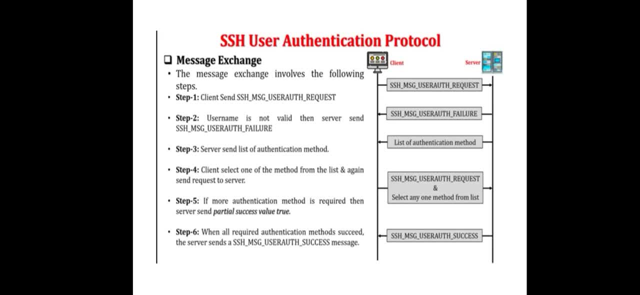 after client authentication request, server check the сердeto user name. if the user name is invalid, server send authentication as fail. user authentication fail message to the client. if user authentication is fail, then server sends a list of authentication method to the client. after that, client send one method from the list. 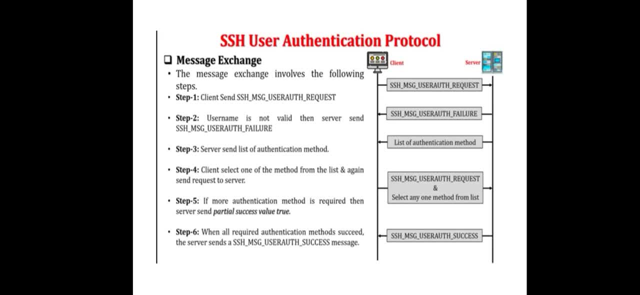 and again send a list ofariamente from the list in the system. send a request to the server. after that, server checks the authentication request. if more authentication required, then servers and partial success values true to the client. when all required authentication method success, then server sends user authentication success message. 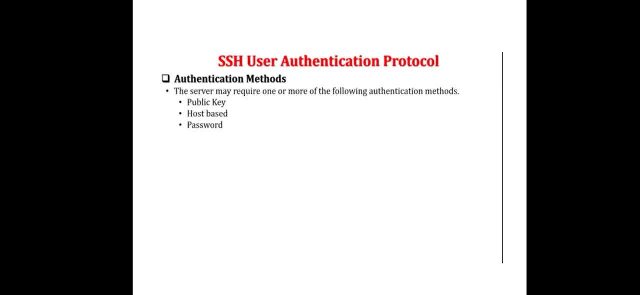 to the client. next one is authentication methods in authentication protocol. in this we are having public key, host based and password. so in public key the message is encrypted by client's private key and client sends its public key to server along with message and server decrypt that message using client's public key and in host based, all the clients. 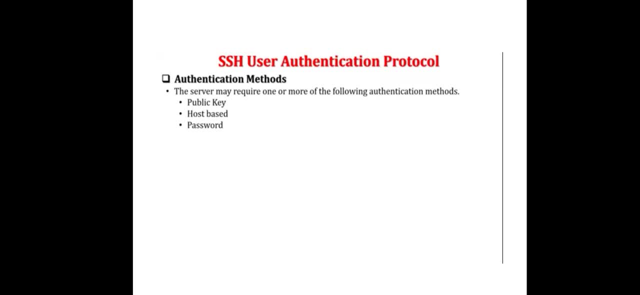 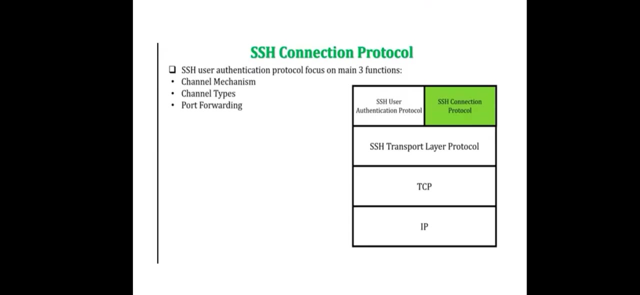 are connects with the central system. it is called as host. host public key is shared with all the clients and password means client sends a message containing a plain password. this message is protected- means encrypted- by the transport layer protocol. and the next protocol is SSH connection protocol. in this connection protocol the three main functions are there. first one: 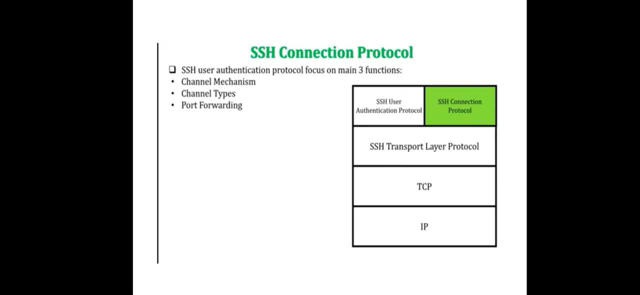 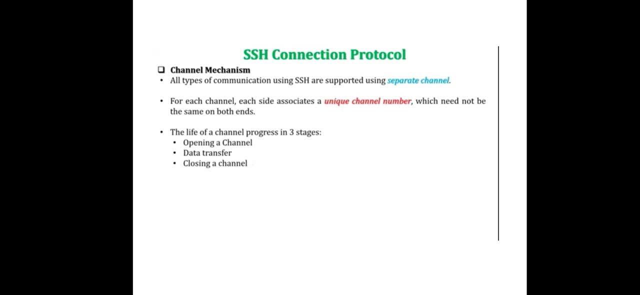 is channel mechanism, second one is channel types and third one is port forwarding. about channel mechanism: let's see about channel mechanism. all types of communication using secure cell are supported using separate channel. in this function, for each channel, each side associates a unique channel number, which need not to be the same on the both sides. it means channel number. 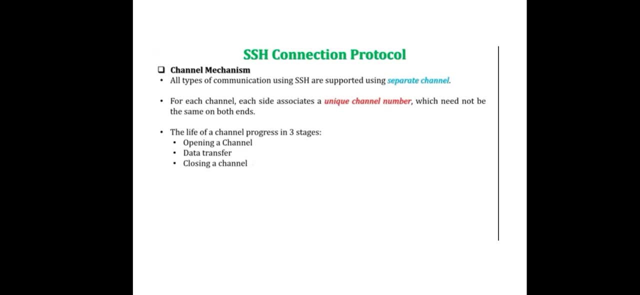 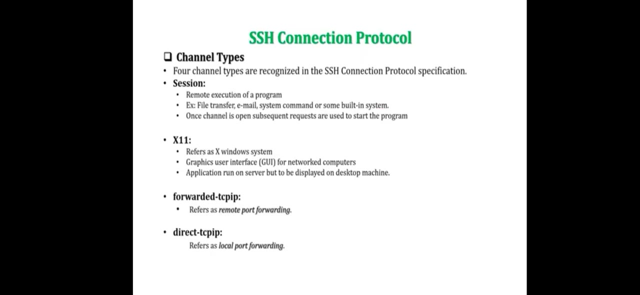 from the side, client side and the server side, both unique. and the last one is the connection between the server and the network and the life of a channel. progress in three stage. first is opening a channel. second is data transfer. third is closing a channel. now, next one is channel types in connection protocol, four channel types. 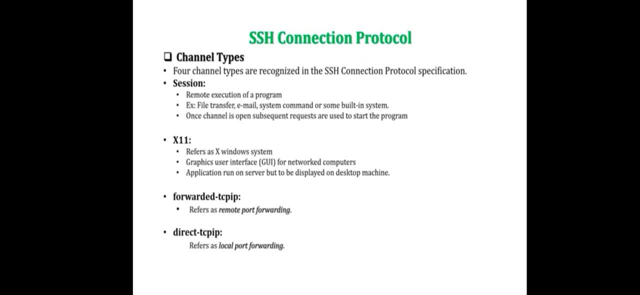 are recognized in the secure cell connection protocol specification. first one is session, second one is x11. third one is forwarded tcpip. fourth one is direct tcpip. so session means this channel is mostly used in remote execution of a program example like email file transfer system, command or some built-in systems. once channel is open, subsequent request are used. 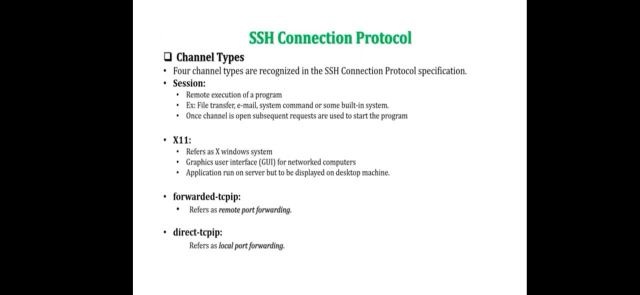 to the start the program. and in x11 this kind of secure cell channel is used in x window systems. this channel proves graphical user interface for network computers. so it means applications. so it means the application run on the server but to be displayed on desktop machine. so these kind of channel mostly used. 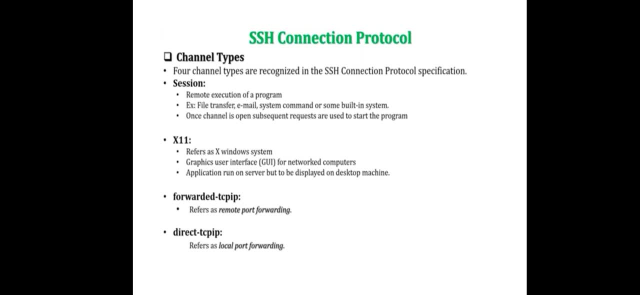 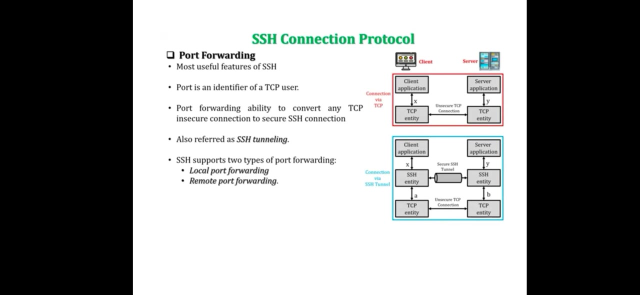 in disturbed network environment and forward tcpip it refers as a remote port forwarding and direct tcpip it refers as a local port forwarding. now let's see about port forwarding in connection protocol. it is most useful. features of secure cell: port is an identifier of a tcp. therefore, the features of ssh is the port forwarding. 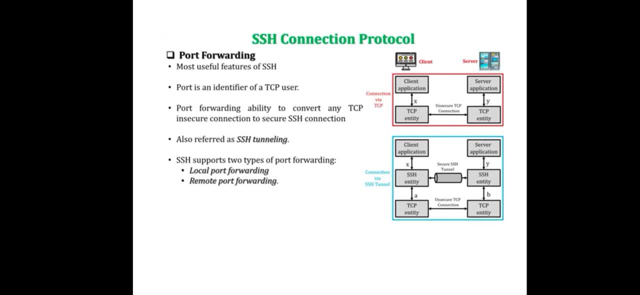 ability to convert any tcp in secure connection to secure ssh connection. it is also referred as ssh tunneling means port forwarding is the most useful features of a secure cell. it means here: secure cell connection means that ssh tunneling is always created between local secure entity and remote secure entity.